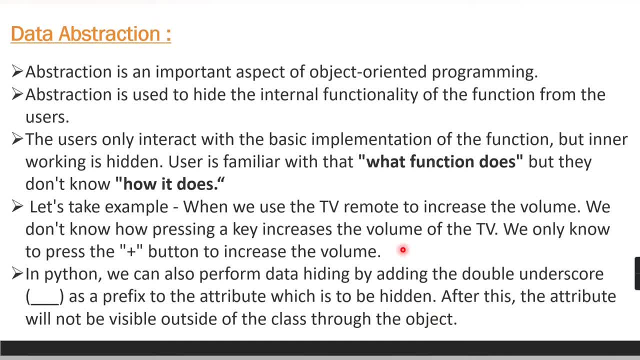 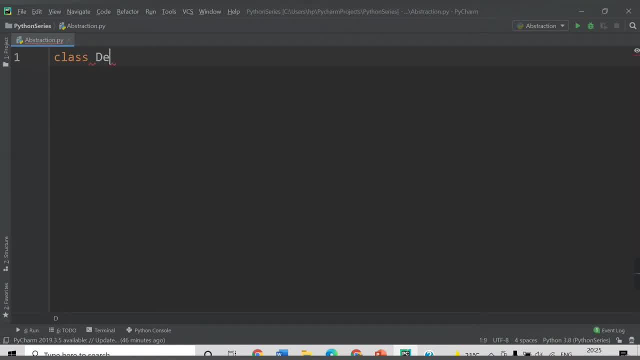 So let's see in our demo how we can achieve the data hiding in Python. So this is my abstractionpython file. So let's declare one class, Let's say demo. So in this class I have two attributes or two variables. Let's say I, which has the value 1, and the second variable I want to hide. 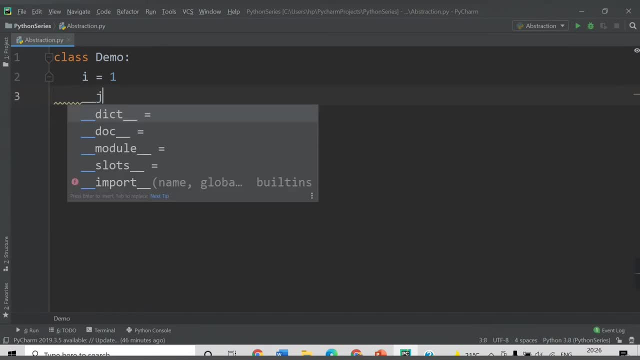 So I will need to provide the double underscore as prefix and the name of attribute, which is j, and value as 2.. So these are my two variables inside the class And I will have one method here: Dev show. So this is the name of the method: show, Sorry, show. 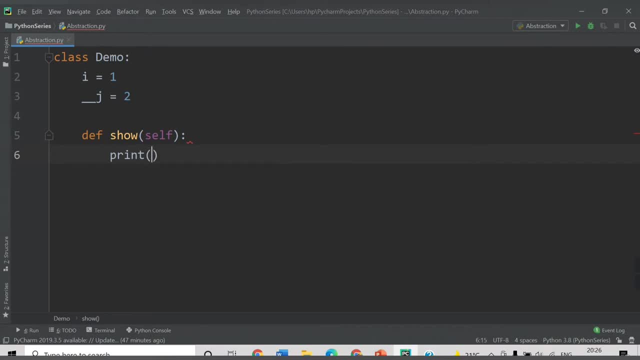 And inside this method I will print Print Value of i and I will have here self dot i. So in this way I can access this variable i. I will copy this statement and in similar way I will say value of j, So value of underscore j, and here I need to say the underscore j. 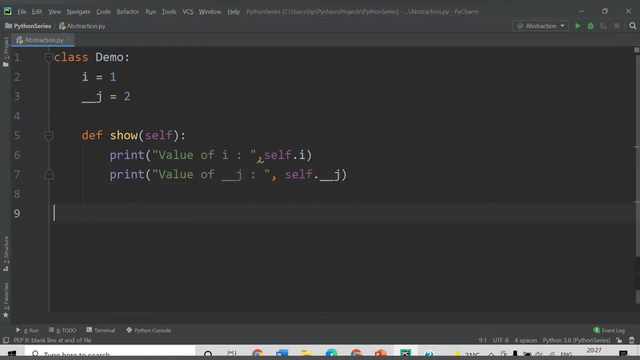 And I will now come outside this class, So proper intonation should be given. So currently I am outside this class now, And here I will create the object of this class. Let's say object is d, d equals to demo, And with the help of this object I will call the method show. 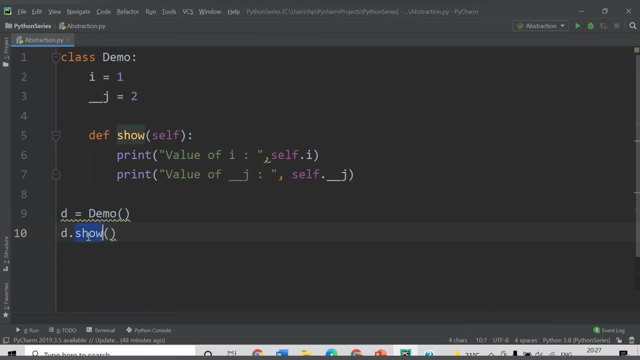 Now what will be the output? The object will call this method show. So here we will get the show. And we will get this: two statements: value of i, Which is one, and value of j, which will be two. Let's run this code. 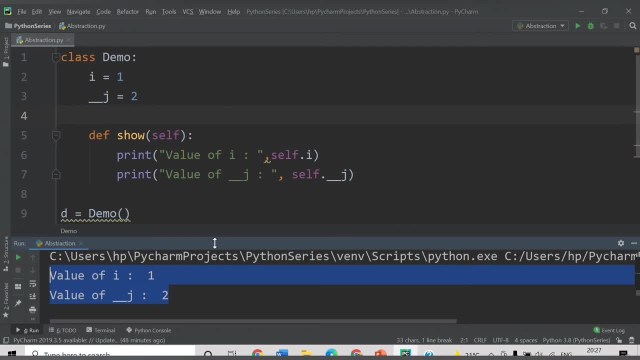 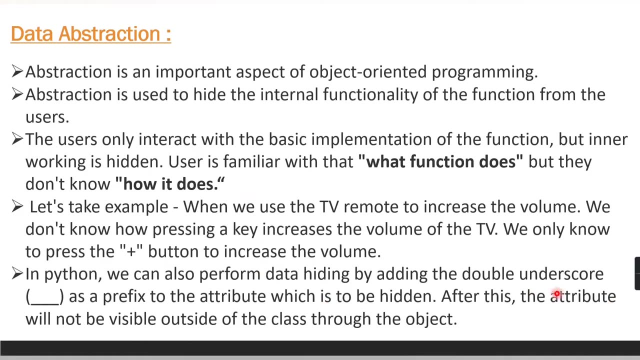 So see, we are getting here value of i as one and value of j as two. So now we want to hide this data, right, j. So what does the theory says? It says the attribute will not be visible outside of the class through the object.